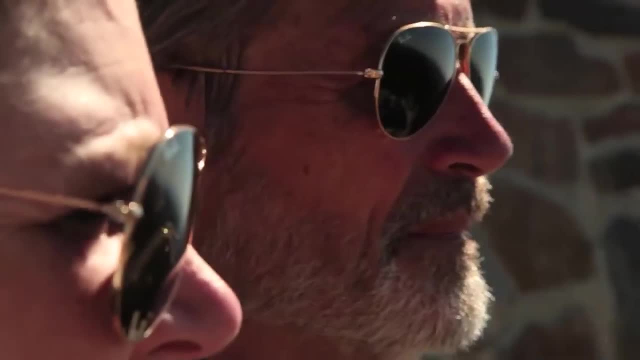 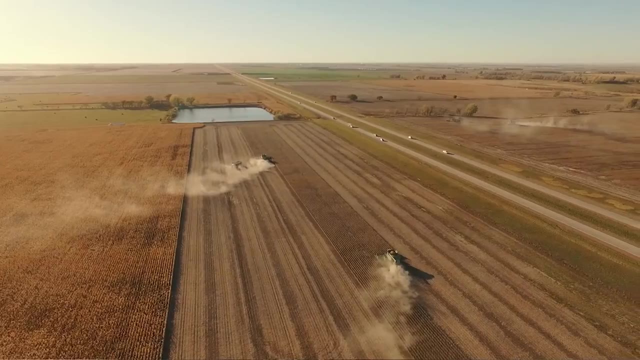 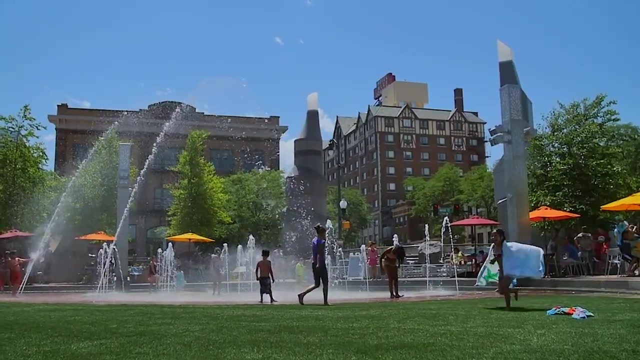 for residents and visitors alike. Today, South Dakota has a population of about 892,000 people. The state has a diverse economy, with significant industries in agriculture, tourism, manufacturing and retail trade. South Dakota is known for its beautiful scenery, with iconic attractions such as Mount Rushmore and the Badlands National Park. 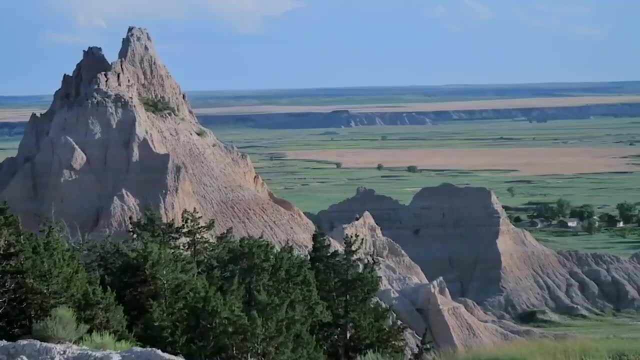 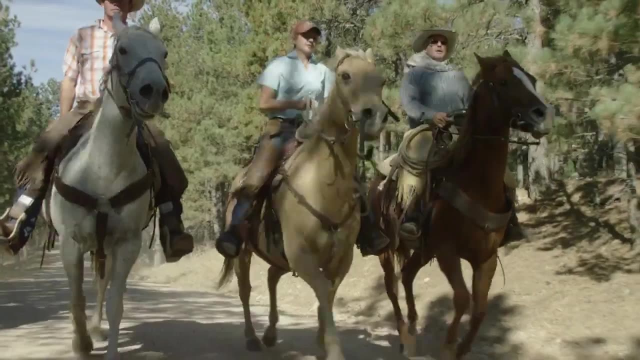 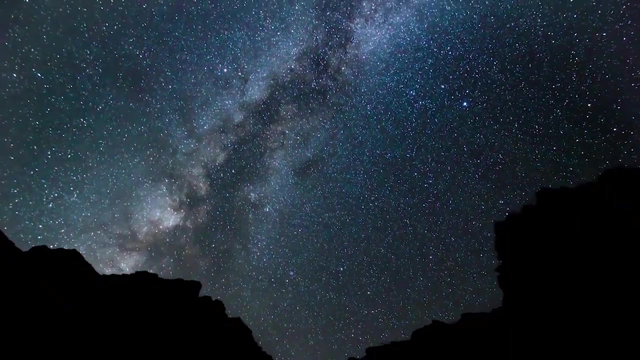 Drawing visitors from around the world. the state also offers plenty of outdoor recreational opportunities, with hiking, camping and fishing being popular activities. Overall, South Dakota is a great place to live and visit, with a rich history, beautiful scenery and a thriving economy. South Dakota was first explored by European. 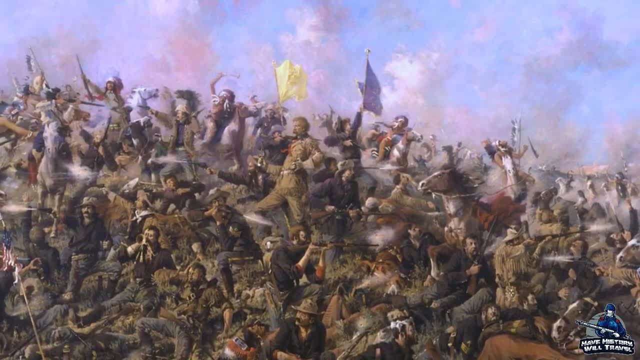 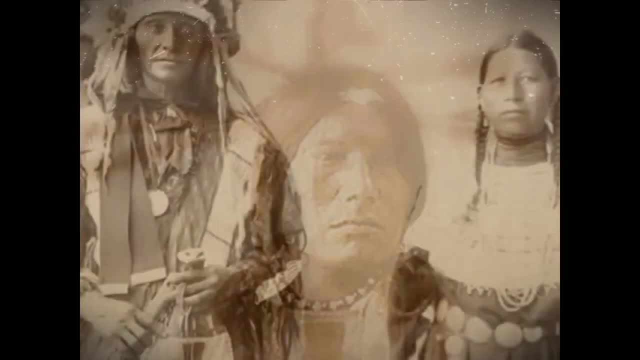 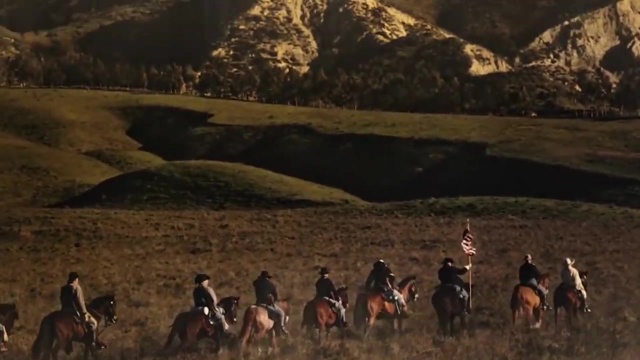 settlers in the early 1800s and it was admitted to the Union as the 40th state in 1889.. South Dakota is home to some of the most famous and iconic attractions in the United States. One of the must-see destinations in the state is Mount Rushmore National Monument, where you can see 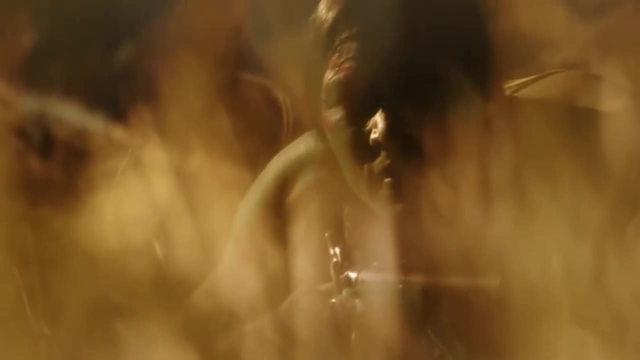 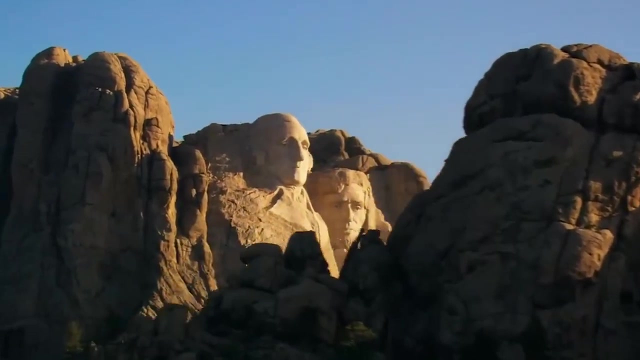 the faces of four American presidents carved into the side of a mountain. This monument is a treasure trove of historical sites and heritage and became one of the top attractions in the United States. It's been a great year in the US since the beginning of the century. 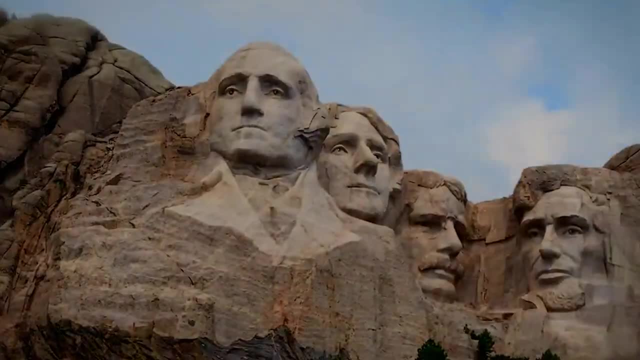 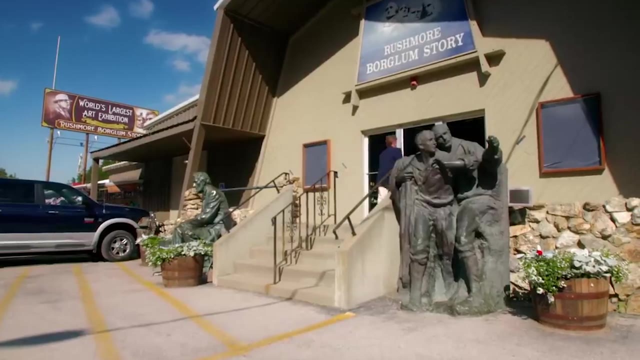 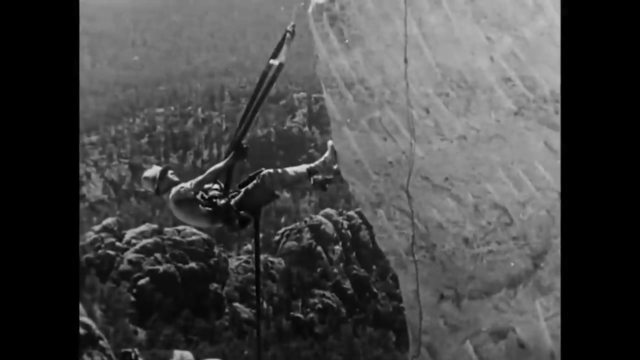 with some of the most famous and iconic attractions being the Black Lives Matter and UNESCO World. This monument is a true American icon and a great place to learn about the country's history. Mount Rushmore was created in the early 1900s as a way to promote tourism in the region. 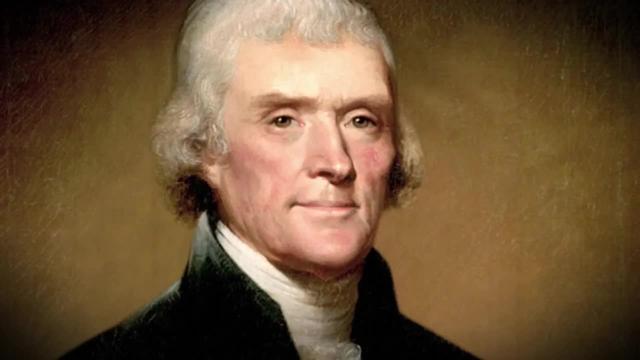 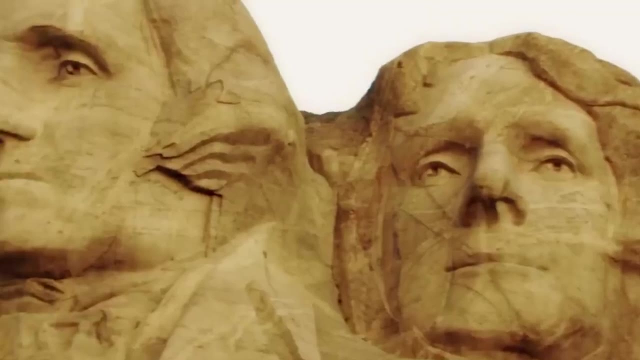 The four presidents depicted on the mountain are George Washington, Thomas Jefferson, Theodore Roosevelt and Abraham Lincoln. These presidents were chosen because they represent the country's founding, growth, development and preservation. Visiting Mount Rushmore is a truly awe-inspiring experience. 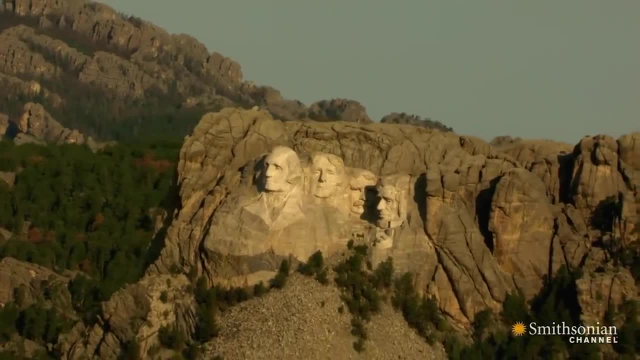 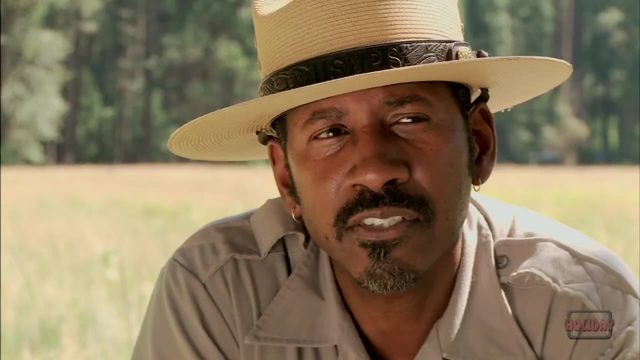 The monument is located in the Black Hills of South Dakota and it offers stunning views of the surrounding landscape. You can take a guided tour of the monument, learn about the history of the area and even take part in ranger-led programs and activities. 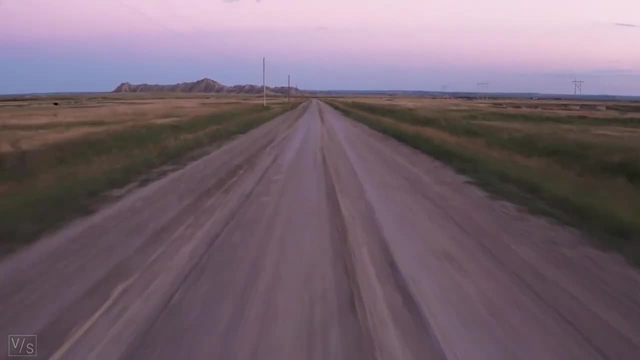 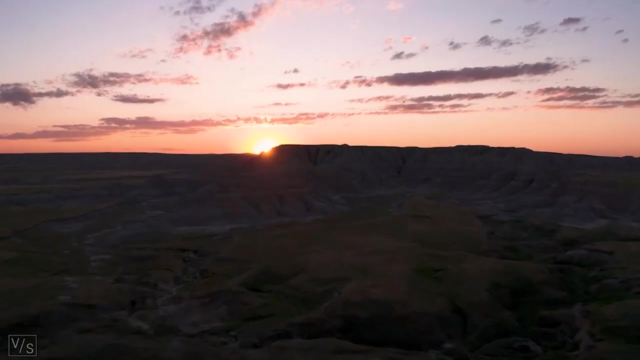 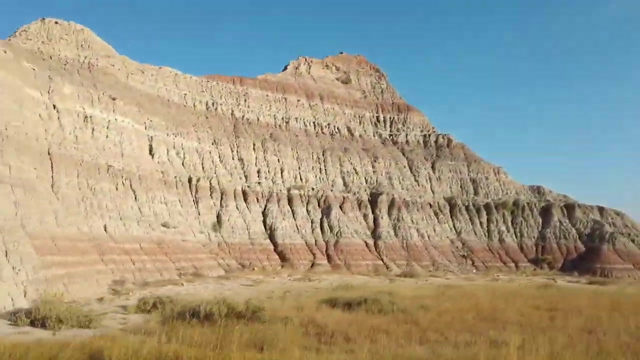 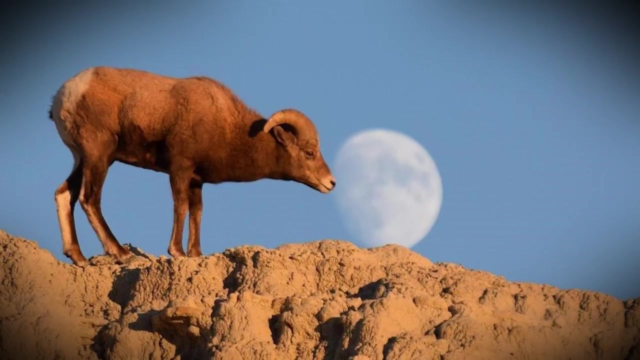 In addition to Mount Rushmore, South Dakota is also home to another famous national park: Badlands National Park. This park is known for its striking landscapes and abundant wildlife, and it's a great place to hike, camp and explore. The park covers over 244,000 acres and is home to a wide variety of plants and animals, including bison, pronghorn and bighorn sheep. 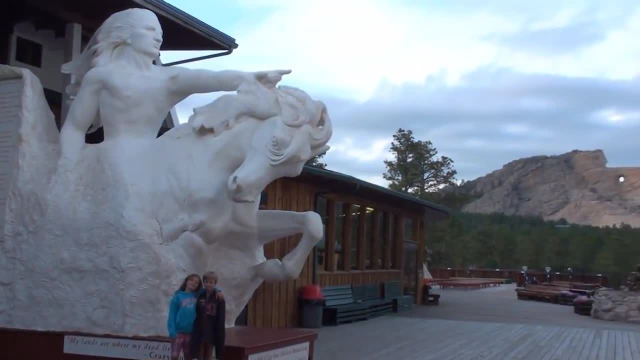 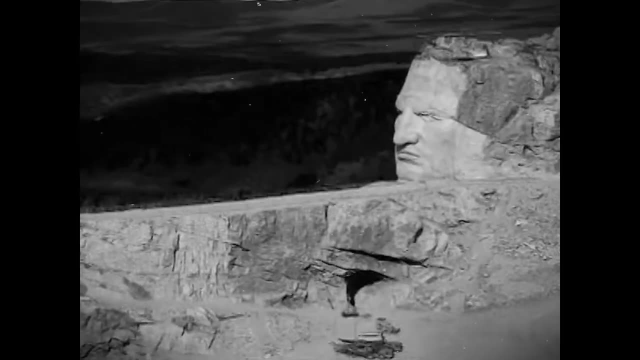 Another historical site worth visiting in South Dakota is the Crazy Horse Memorial. This memorial honors the famous Lakota warrior, Crazy Horse, and it is still being carved into the side of a mountain. The monument is a tribute to the Native American culture and history of the region. 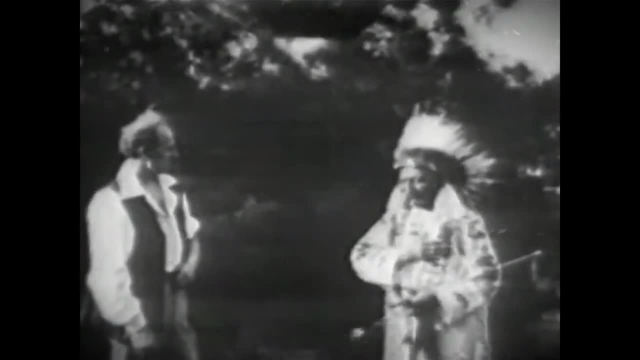 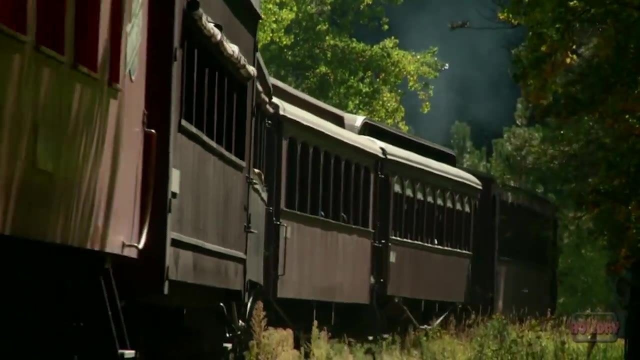 and it offers visitors the chance to learn about the history of the region. If you're looking for a truly unique experience, take a ride on the 1880 train, a historic steam train that takes passengers on a scenic journey through the Black Hills. 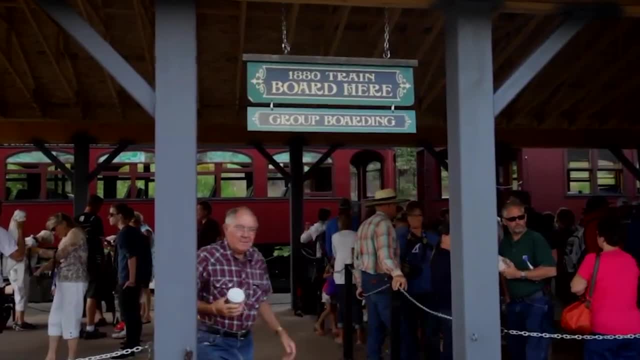 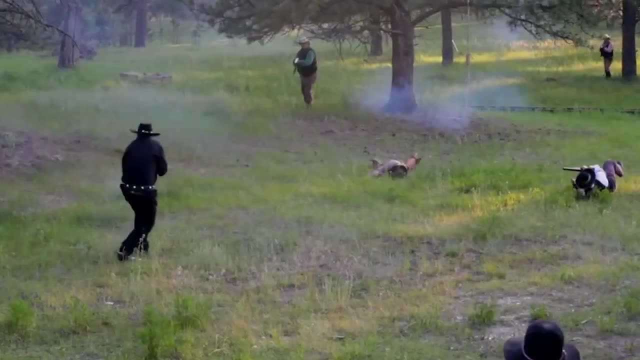 This is a great way to see the beauty of South Dakota and learn about the state's history. at the same time, The train offers regular departures from Hill City and it's a fun and exciting way to explore the state. Overall, South Dakota offers a great mix of life and adventure. 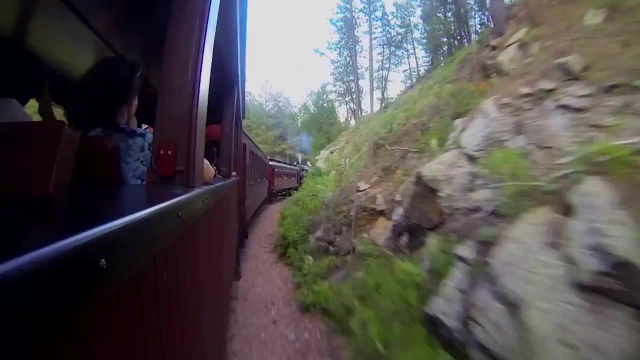 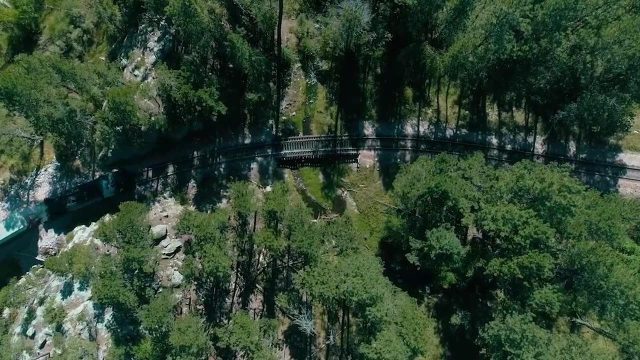 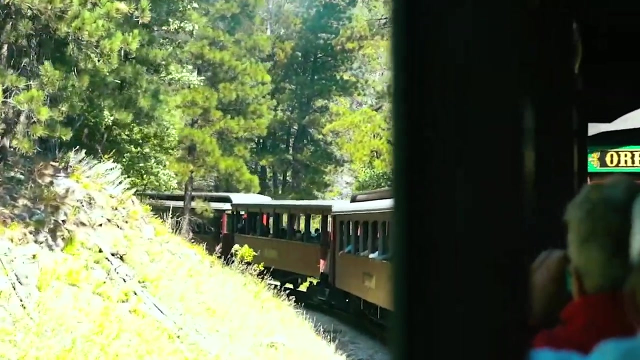 It has a great mix of natural beauty, history and unique attractions. Whether you're looking for outdoor adventures, cultural experiences or just a chance to relax and enjoy the scenery, South Dakota has something for everyone. So why not plan your next vacation to this beautiful state and see for yourself what it has to offer? North Dakota has a population of about 762,000 people, and its economy is focused around industries in agriculture, tourism and tourism. The state is known for its natural beauty, with the Theodore Roosevelt National Park and the North Dakota Badlands being popular destinations for outdoor enthusiasts. 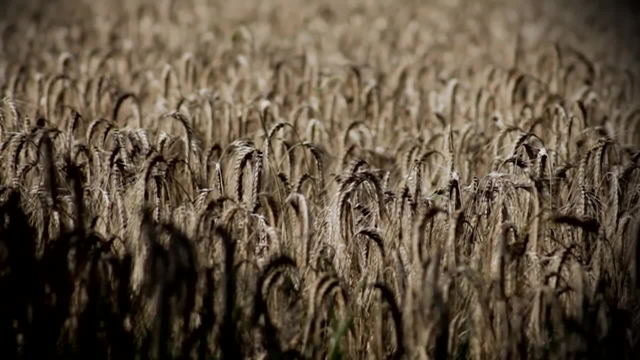 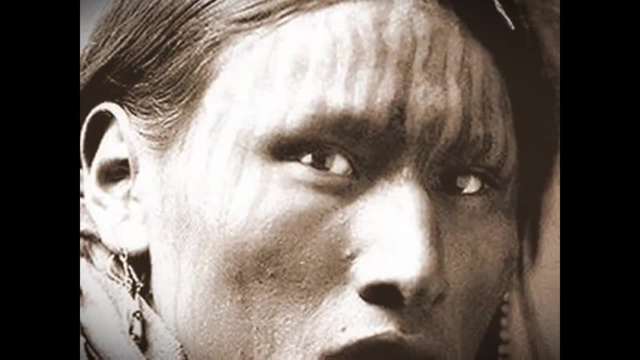 North Dakota was also first explored by European settlers in the early 1800s and it was admitted to the Union as the 39th state in 1889.. The state's name also comes from the Dakota Sioux Tribe, who were the original inhabitants of the region. 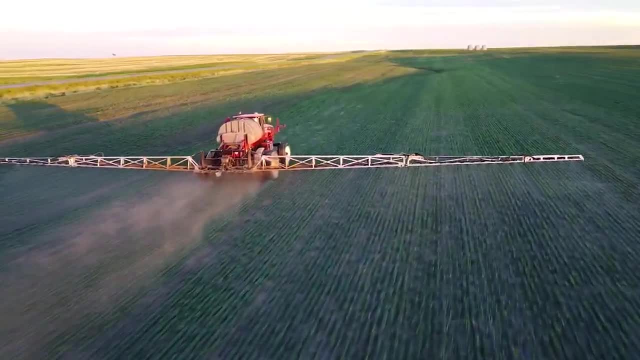 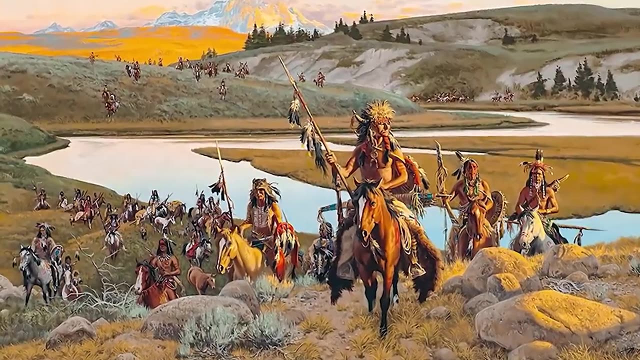 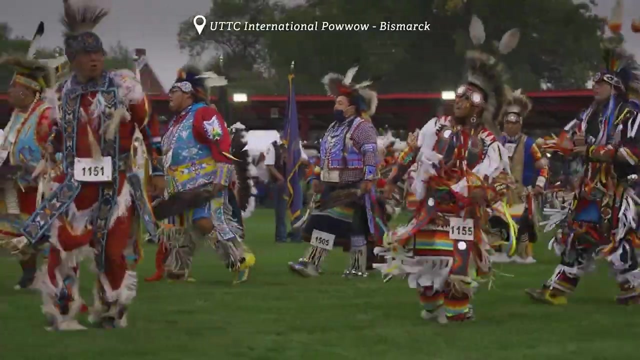 North Dakota has a rich history of agriculture, with the state playing a significant role in the development of the United States' farming and ranching industries. The state also has a rich history of Native American culture, with several tribes calling it home Today. North Dakota is also known for its beautiful scenery, rich history and outdoor recreational opportunities. 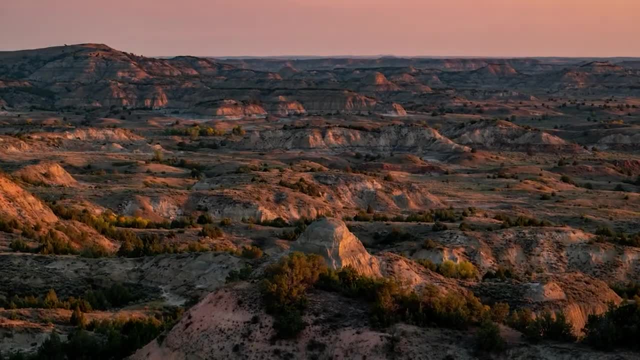 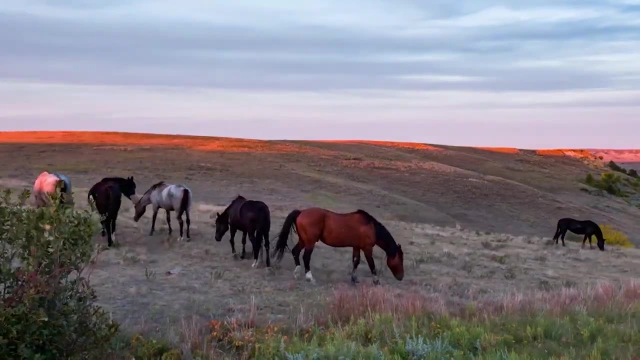 One of the must-see attractions in the state is the Theodore Roosevelt National Park, named after the 26th President of the United States. This park offers beautiful hiking and camping opportunities, scenic trails, scenic drives and the chance to see bison and other wildlife. 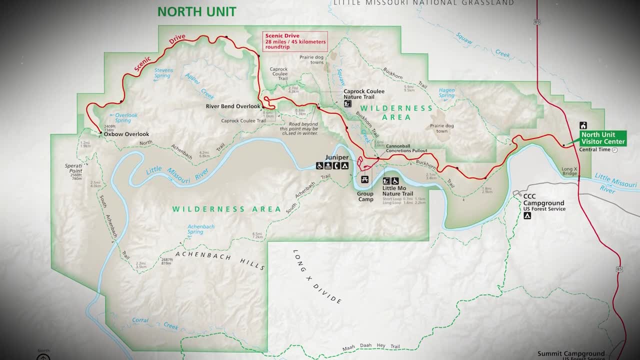 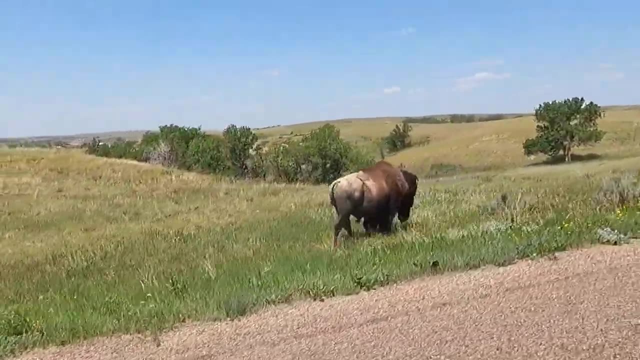 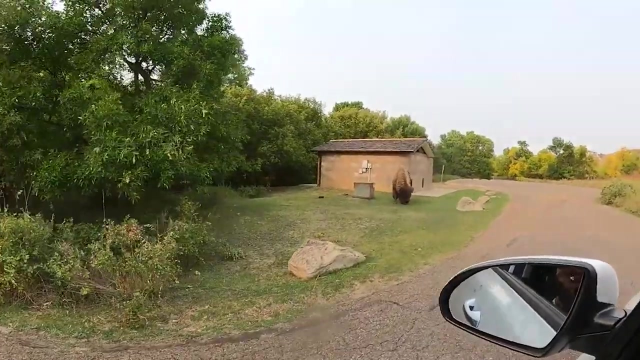 The park is divided into three units, each offering a different experience. The North unit is located near Watford City and offers scenic drives, hiking trails and the chance to see wildlife. The South unit is located near Maduro and offers similar activities, as well as a visitor center and a scenic overlook. 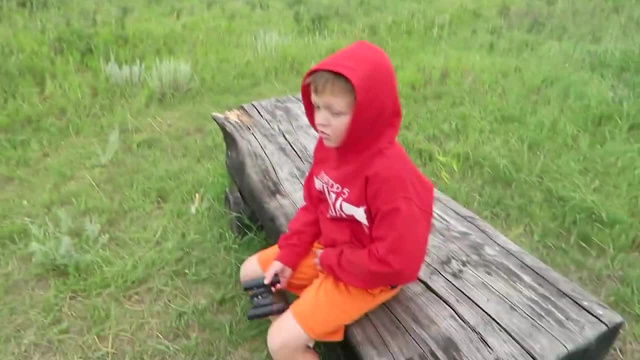 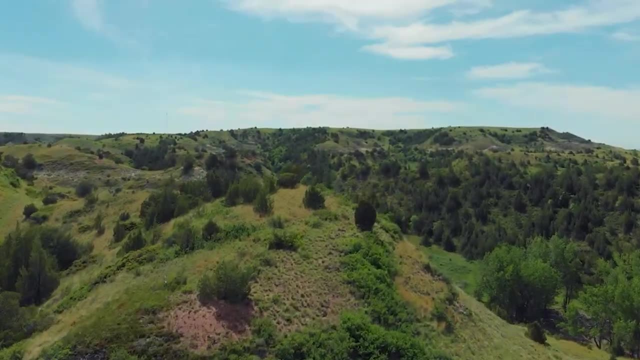 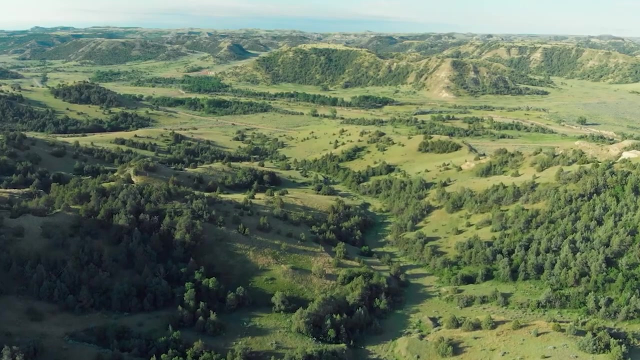 The Elkhorn Ranch unit is only accessible by hiking or horseback riding and offers a more remote and rugged experience. Another great destination for outdoor enthusiasts is the North Dakota Badlands. This area offers beautiful hiking and camping opportunities and it's a great place to explore the rugged beauty of the state. 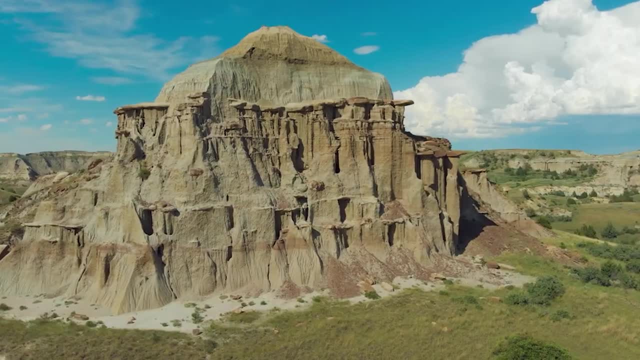 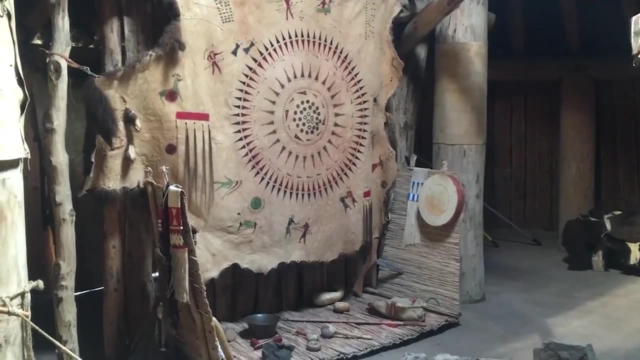 There are several state parks and recreational areas in the Badlands, including the Knife River Indian Village's National Historic Site, which offers the chance to learn about the history and culture of the Hidatsa, Mandan and Arikara tribes. 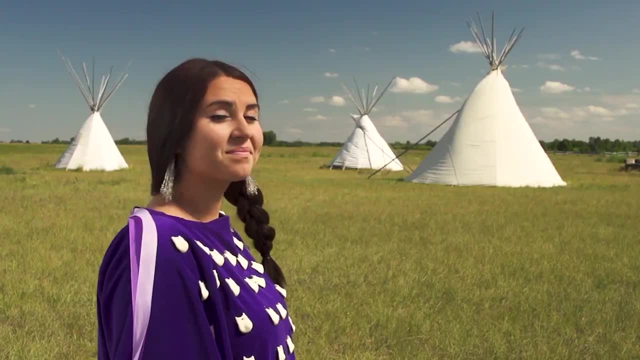 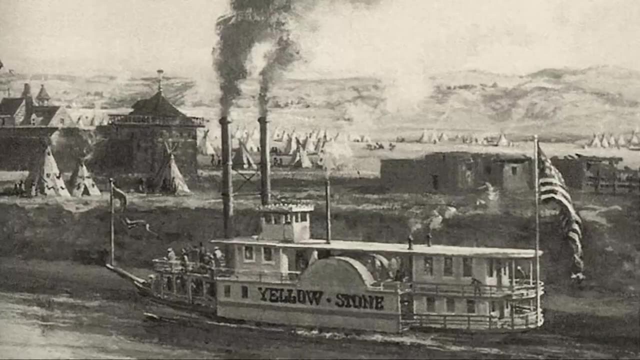 For those interested in North Dakota's history and culture, there are several interesting attractions to visit. One of these is the Fort Union Trading Post, a historic site that was built in the 1800s and served as a hub for trade and diplomacy between the United States and several Native American tribes. 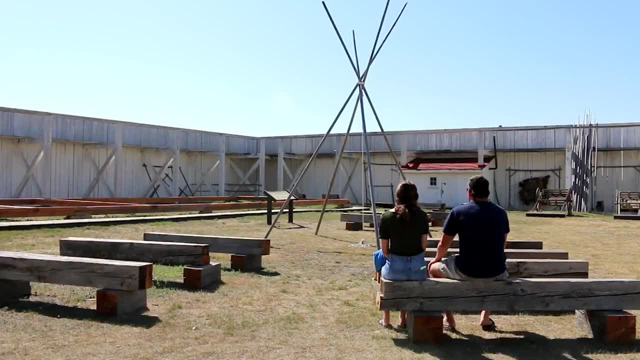 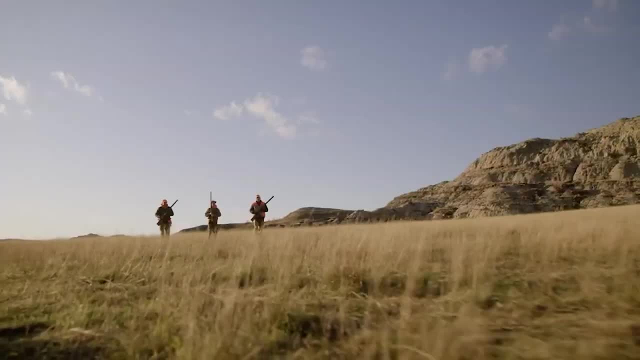 Today the fort is a National Historic Site and offers visitors the chance to learn about the history of the region. In addition to these attractions, North Dakota also offers plenty of opportunities for outdoor activities. The state is known for its excellent tourism, excellent hunting and fishing. 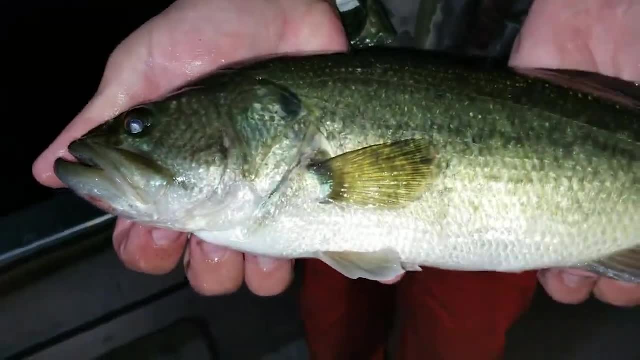 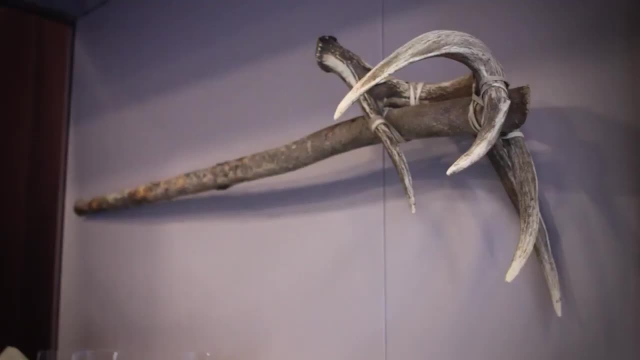 and there are plenty of opportunities to catch trophy-sized game and fish. North Dakota also has a rich agricultural heritage, and visitors can learn about the state's farming and ranching history at the North Dakota Heritage Center and State Museum in Bismarck. 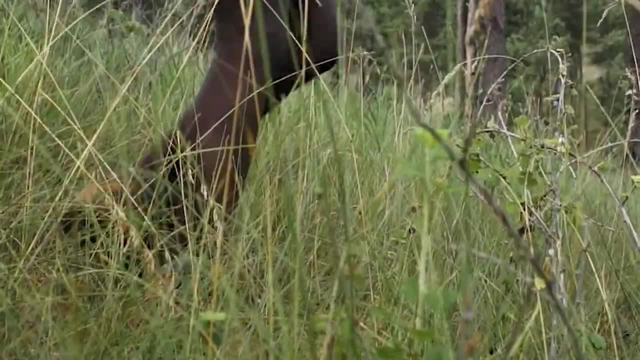 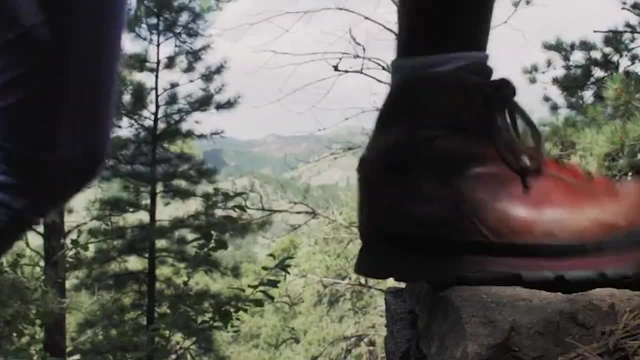 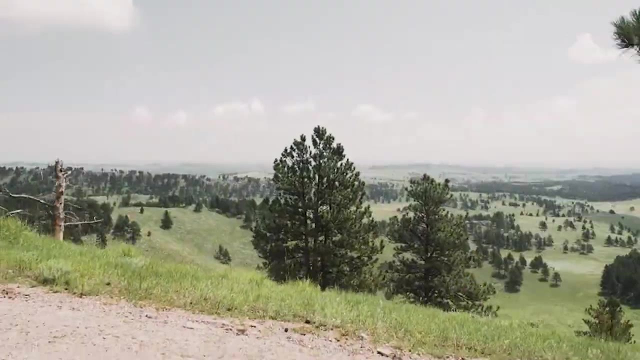 Overall, North Dakota is a great destination for those looking to explore its natural beauty, history and culture. Whether you're interested in outdoor activities, historical sites or unique cultural experiences, North Dakota has something for everyone. So why not plan your next vacation to this beautiful state and see for yourself what it has to offer?